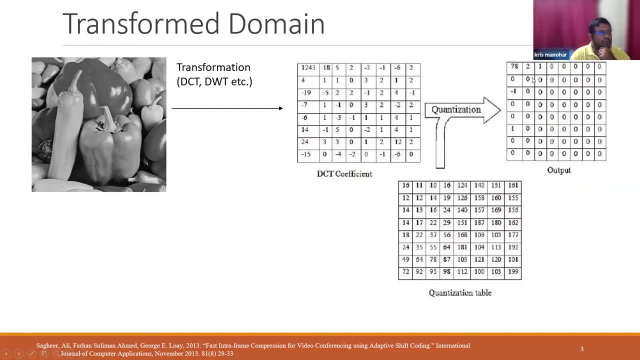 quantization table. um you, you focus really just on the important components of that signal and you have a lot of this redundant space, right. and then this space now is what is um usually entropy encoded. so they would do a sort of zigzag type scan and it would generate a 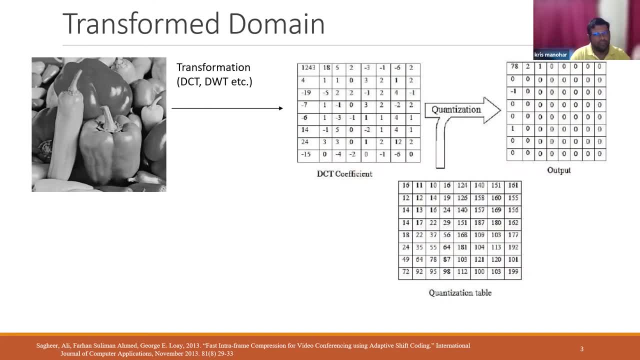 uh, sequence with a lot of repeats, and then they'd use, like a move to front technique, to, to, to reduce the, the um number of bits required to represent that information further, right? so what they would do then is when they, when you're reconstructing now, um, these, when they take, 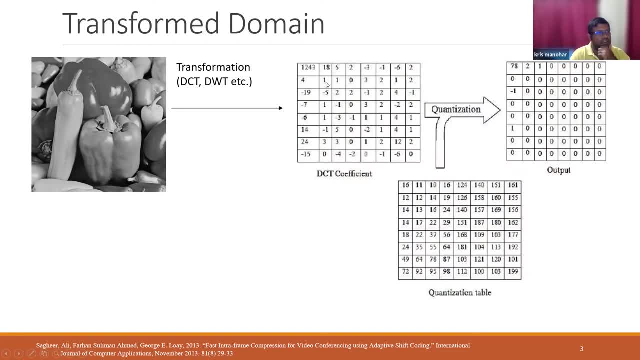 these coefficients. they multiply by these stuff in the quantization table, they get something that's approximate to the original dct representation- anything right. so that's typically how it goes. from the transform they mean techniques work. so what they would usually do is that they would try to modify these coefficients here right after the quantization step in a way that 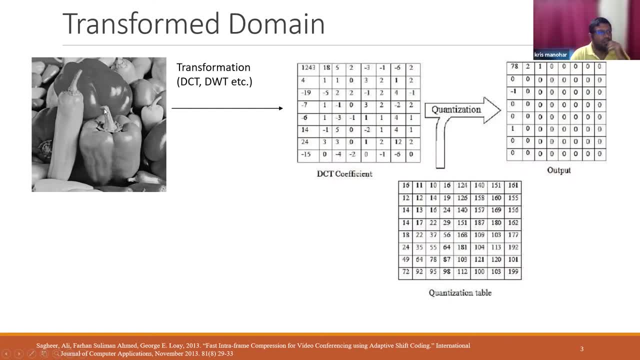 would minimize the overall distortion in the image, right, but a lot of the techniques, they didn't really look at the file size as well, right? so now we have like sort of three competing um three, three competing objectives here, right? so you want to maximize embedding capacity, you want to minimize distortion and then you want to minimize file size, right. 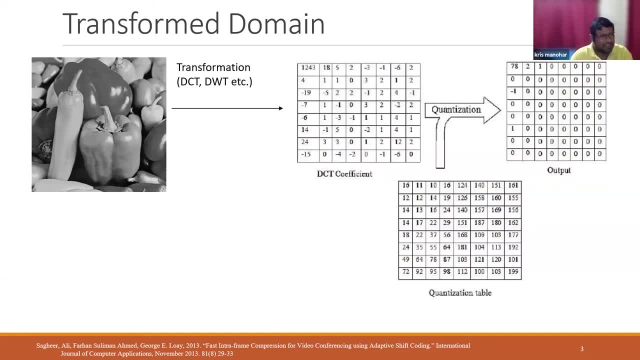 so that was the first interesting thing about this work, this paper. that that caught my eye was that um, nobody ever considered the file size in any meaningful right. so what they did was they. they took this now and they sort of generalized it. so all right, so the, the um. 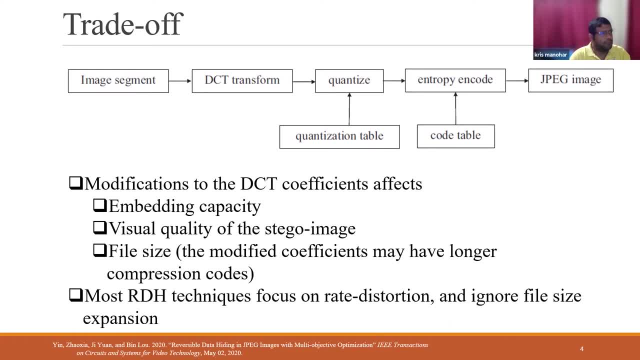 the general framework for the transform. the main techniques is they have this information segment, you bring it in here, you work out the transform, then you quantize and then you entropy and code and that's where you get the image right. so obviously any change right, any change in any. 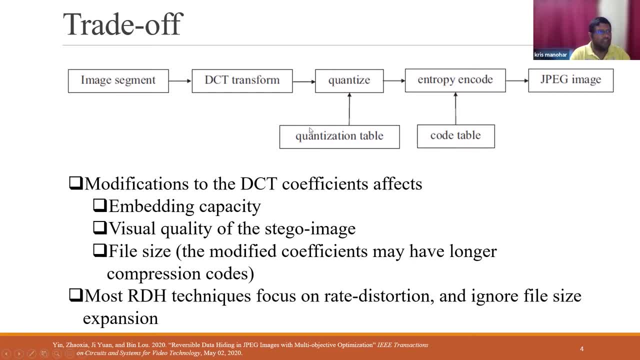 of those coefficients would have an effect into the file size. so because of the increase in the file size, it may introduce embedded capacity, depending on how the coefficient is modified, because sometimes changes have to be made so that the original coefficients could be recovered, right um so they don't embed any secret bits with that. 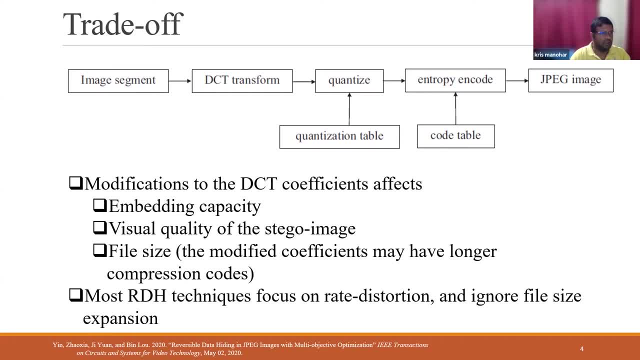 particular change right, and some of them, they, they can um those changes. so two purposes: one to hide secret information or cause also also enable you to massively right. so so that's the general general um. So once you change something in the codes here, then you know we have this sort of effect. 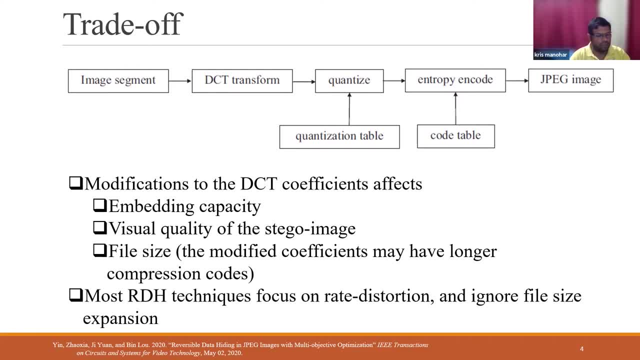 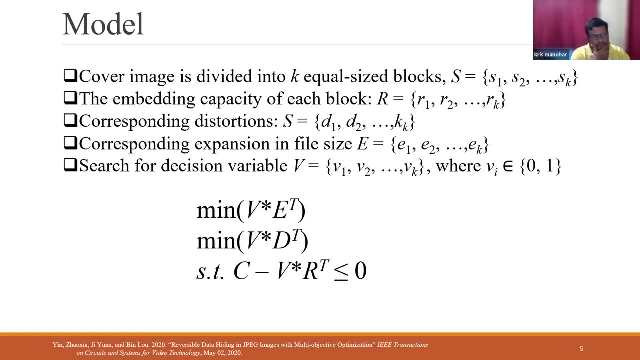 between visual distortion, embedding capacity and files. So how they put all of this together, their model. now they say, okay, well, they have this input signal, which is this image. You divide it up into several equal size blocks, So that'll be a set S. 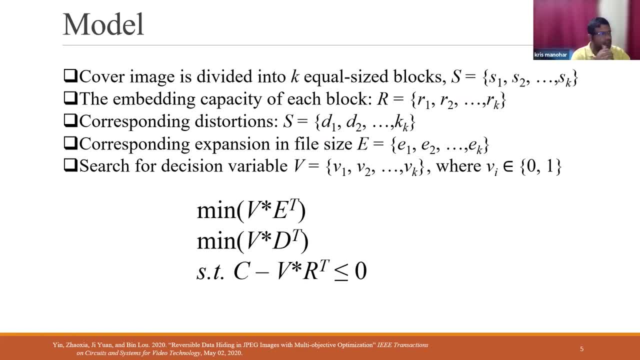 So SI is a particular block, usually eight by eight right. Then the embedding capacity represent that, as you know. so this embedding capacity here for each block kind of depends on the reusable technique that you're using, right? So depending on the algorithm that you're modeling here, 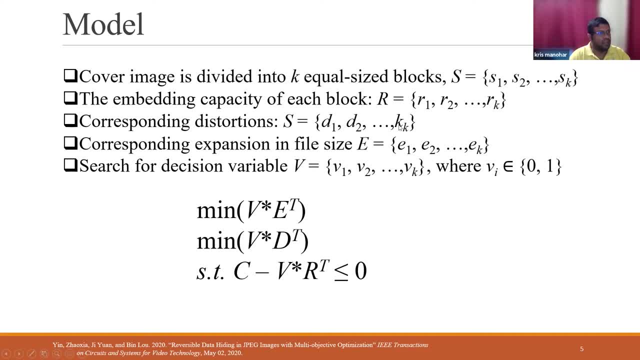 this would have different values. Then, of course, for each particular- oh, this should have been D. Yeah, then for each particular block. I doubt it used some sort of distortion right, So it should be D here, not this right. 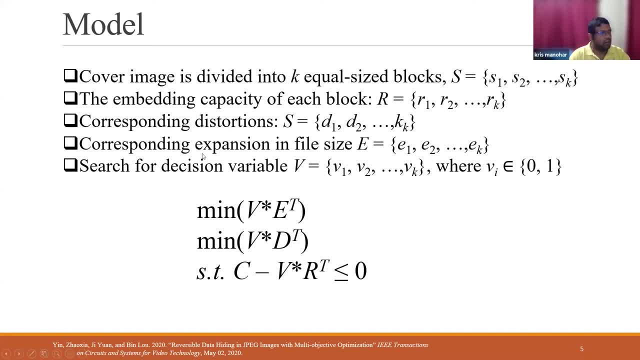 And then the corresponding file size expansion would work Right. So basically, what you'd want to do is you'd want to, you'd want to minimize the overall. So if we were to select, so this vector V here would be a decision variable that would determine. 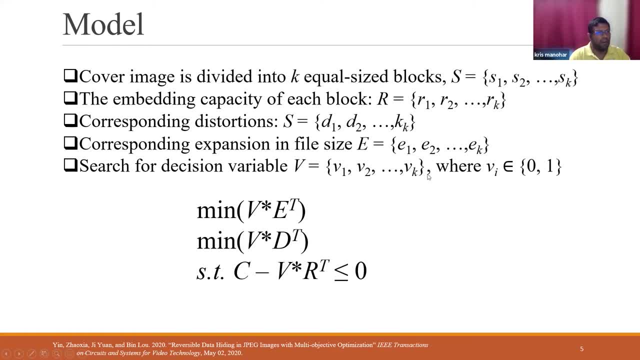 whether or not you select to use a particular block under a reusable data hiding technique, right. So, depending on the blocks that you select, right, those would be one. the rest would be zero. So if we multiply that by the pre-configured expansion, 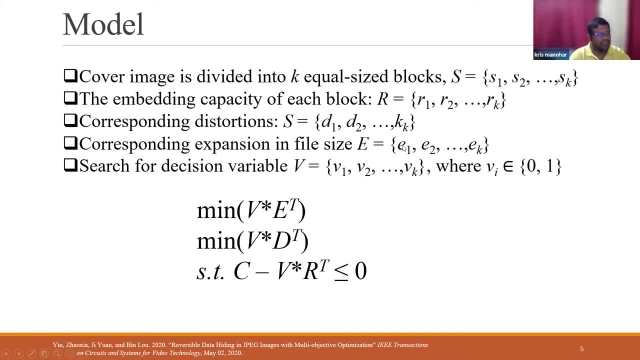 file size expansions for each of the blocks. So these are the increased in terms of the file size that each block, when modified, would contribute. right, So we do that. we will get the total file size and then we can compare that to the original. 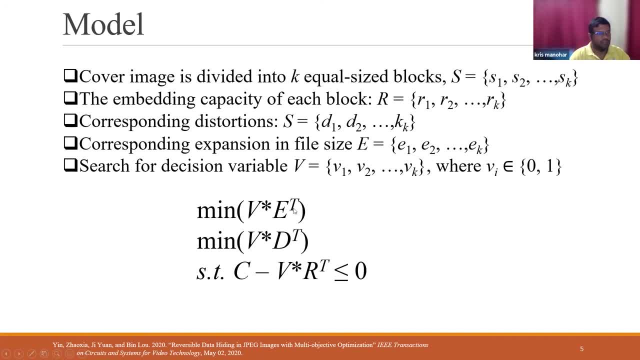 to get a difference right And then, similarly to the distortion right. If we pre-compute that, then we can figure that out And of course we would want the overall embedding capacity right. You want to have enough capacity C such that if you 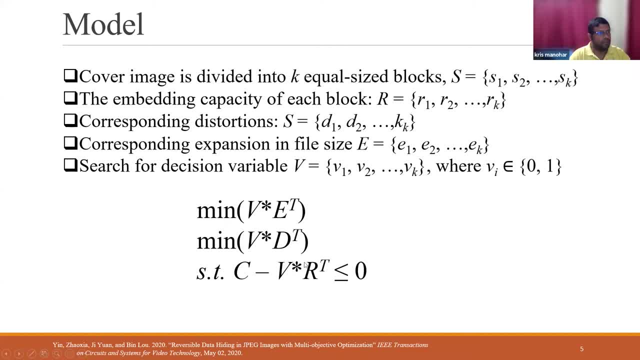 you would to look at all of the bits that you could hide, then you have enough space. So, for example, if C is 10,000, we would want to select enough blocks such that we could hide 10,000 bits, right. 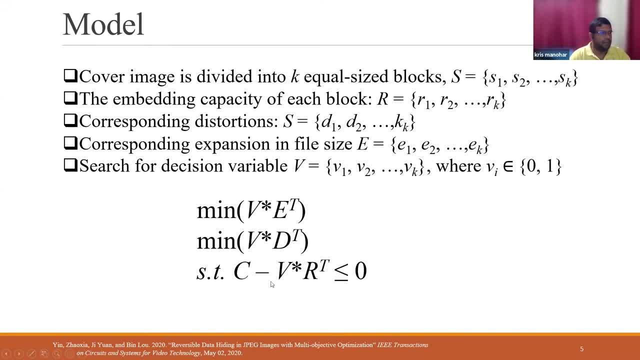 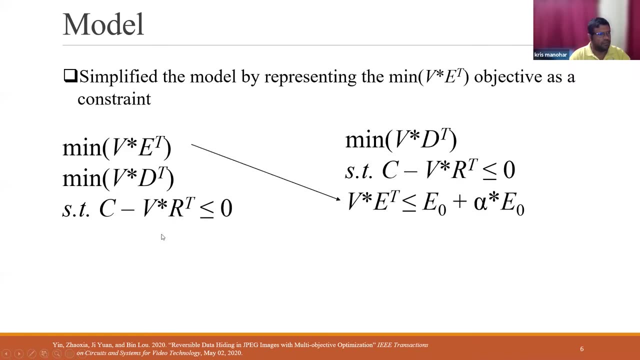 So in other words, the desired capacity. when you take that away from the amount of things that you embed in, you should get something less than zero. So based on that now, we have two sort of objectives here, in terms of the file size and the distortion. 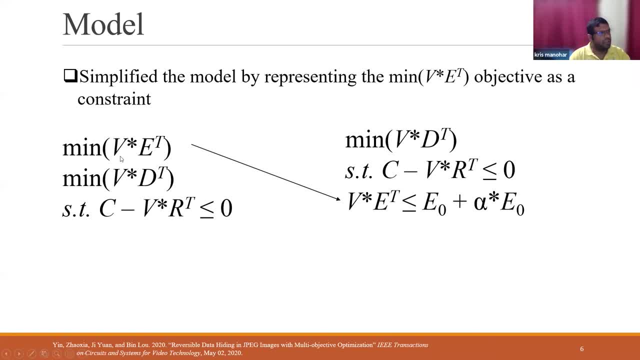 that we'd want to minimize. So, moving on now, what they did was to simplify the computations for this optimization problem. they decided to model the file size expansion as a constraint right. So essentially, what they're trying to say is they want to limit the amount of bits that the image 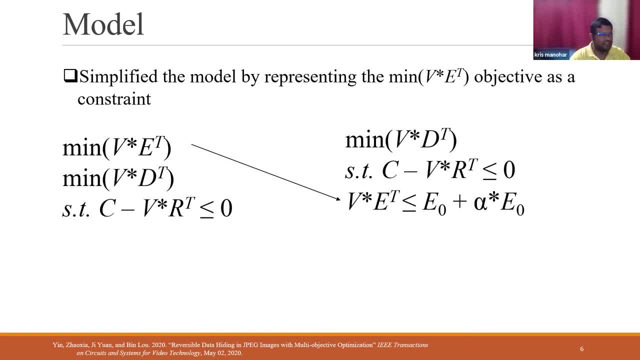 that you produce the cycle image can be bigger than So. it shouldn't be twice as big, It could be probably 1.5 times or maybe just a couple of kilobytes. So that's a parameter, that sort of finds you. 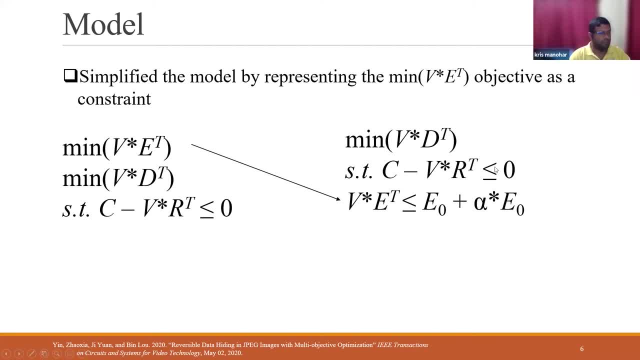 And then, of course, we're doing all of that again by making sure we have enough embedding space to carry all the desired message as well as to minimize the overall stuff, right? So that was the setup. So from here now, this is a much simpler problem. 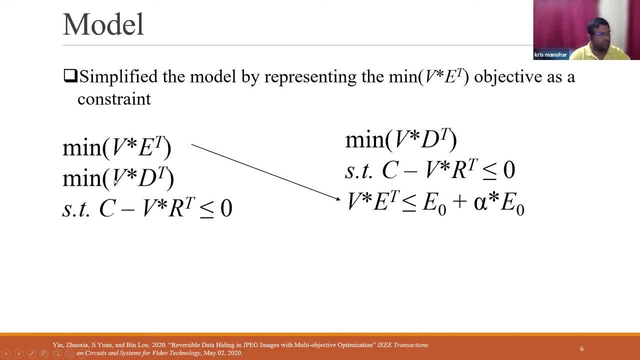 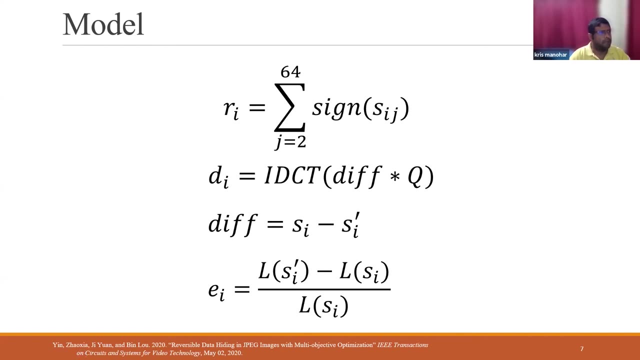 to solve than this one where we have two objectives to solve for here. Here we just simplify by making one another constraint and then we get to solve for the variable b there, right? So in terms of setting up the problem, specifically the RIs, how they would be considered, 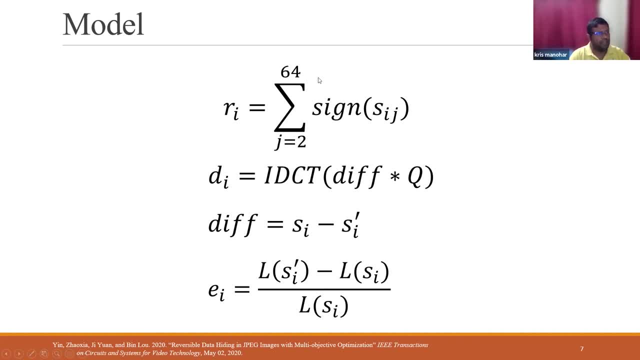 So you would have this coefficient matrix right For the usually eight by eight, so it tends to be 64. This skip the first coefficient because there's a DC coefficient, At least under the discrete cosine transform. that coefficient carries the most spatial. 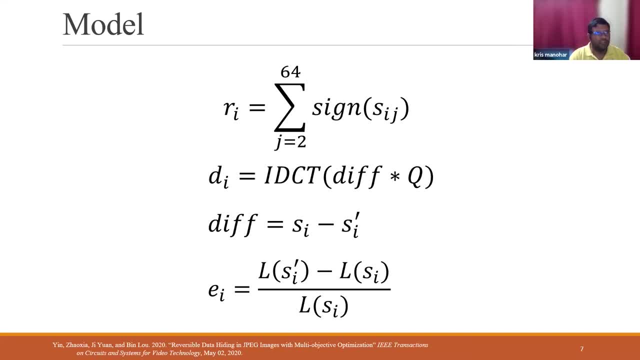 amount of spatial information. So if you were to modify that coefficient, you would see a huge change. So if you were to modify that coefficient, you would see a huge change. So if you were to modify that coefficient, you would see a huge change. 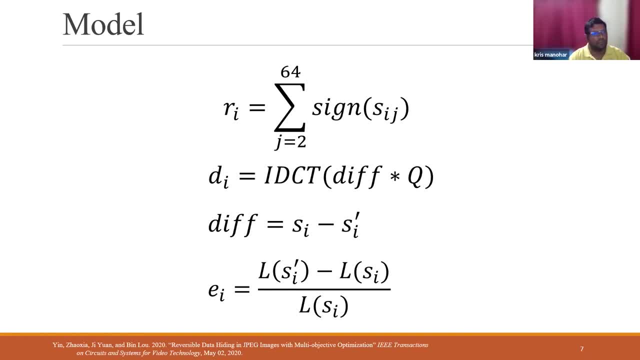 in the visual quality of the image. Typically, the first coefficient in the matrix is left, untouched Right. so that's where we go from two to 64. So essentially, if we are using that particular coefficient in some way, it's the idea is that it would carry. 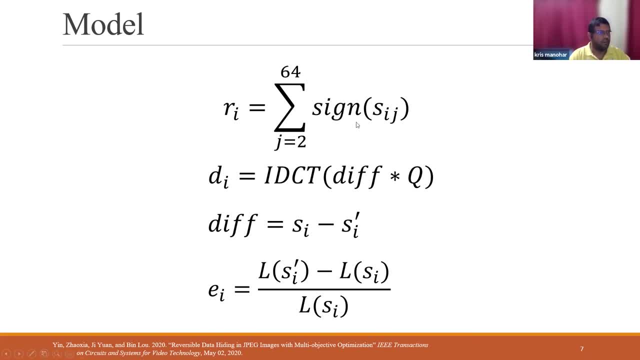 some secret information, right? So we just sum all of the things that we're using. So this sign here will either be zero or one, depending on whether that particular coefficient is embeddable right, In other words, has the ability to carry. 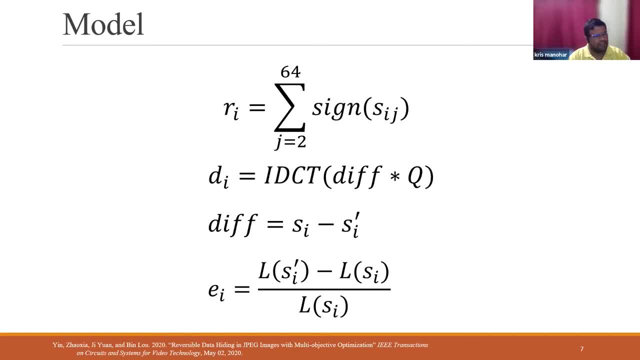 some secret information. So they sort of modeled this after histogram shifting based techniques, right. So with the histogram shifting techniques the maximum bed capacity per pixel would be one bit right Now. it doesn't really generalize to all of the theoretically possible irreversibility hiding techniques. 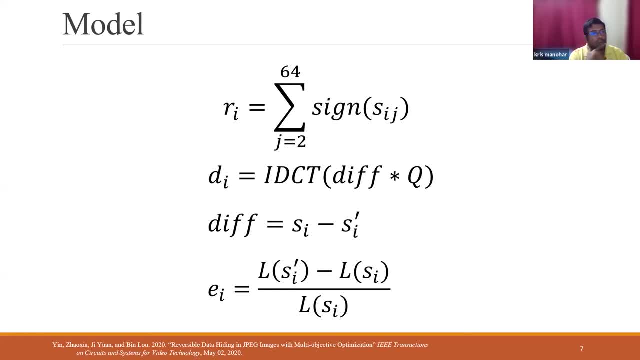 because it is possible to have one coefficient carrying more than one bit right. But in that case the sign function here would just change and you would just associate the number of bits that one pixel would carry right. So that should still work. 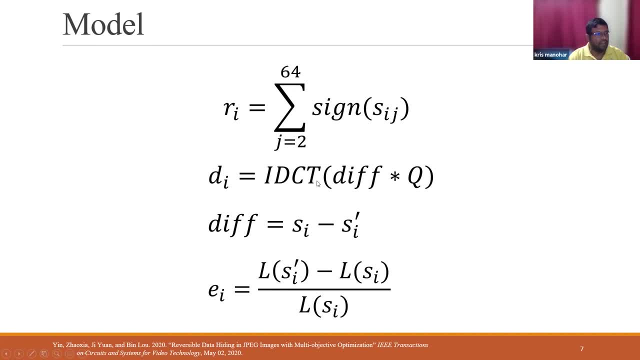 In terms of the distortion, how they would work that out, is it basically? is the IDCT function, That's the inverse DCT where, given the quantized coefficient, you can then get mapped back down to the spatial domain, right? So basically you would just take the estimate. 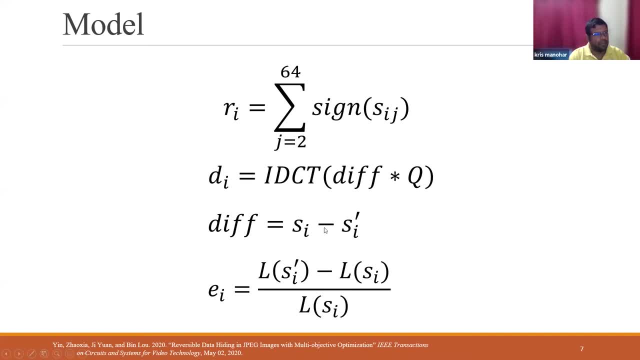 that whether there was a difference between the two In the pixel blocks, right? So this is the coefficient, So SI and then the SI prime is the one that they embed into. So you take the difference between the coefficients and you re-quantize it and pass it through the inverse DCT. 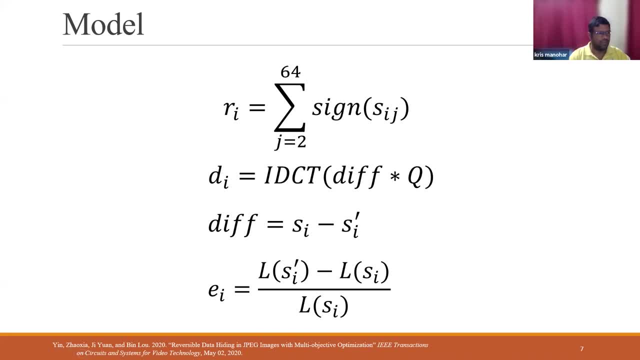 and you would get an estimate as the distortion that would happen there, right. So they modeled it like that. And then, finally, in terms of the size expansion, the EI. how that would work is for Well, encoding JPEG images- at least they use. 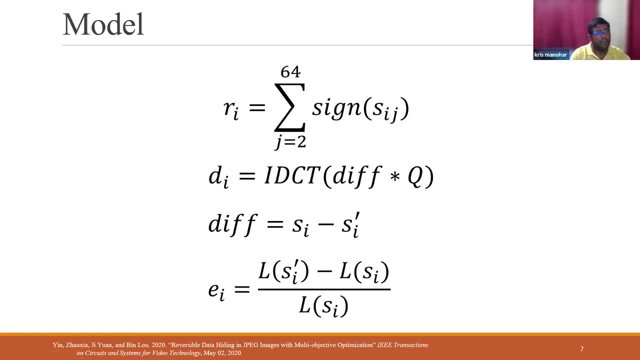 So they do this exact scan and then they move to front, And then on top of that now they would apply a Huffman coding or any type of entropy code at that point right. So usually they would have a table, a Huffman table. 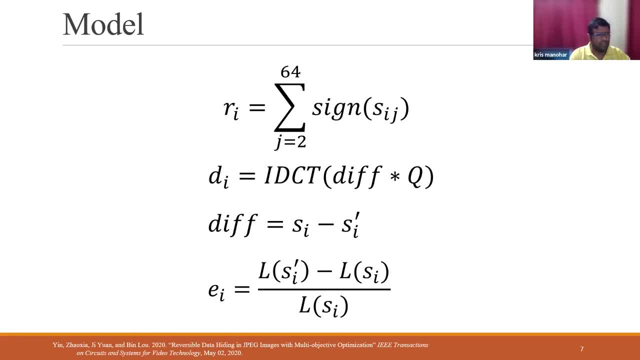 that would be designed that would be associated with a particular quantization table, Because, depending on the quantization table, that affects the coefficients, And then based on the coefficients that would affect the- Yeah, The probability distributions for the different numbers, that you might get like a lot of 0s or 1s or 5s. 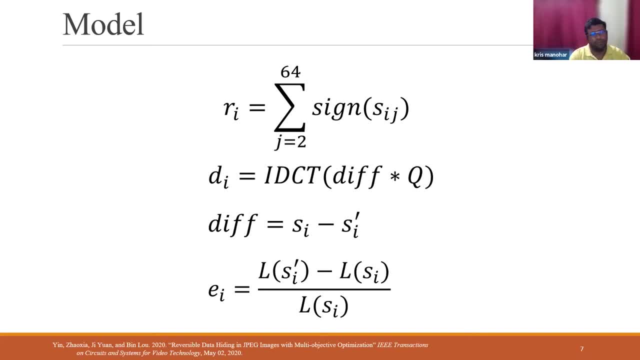 or things like that, which would then affect the Huffman table that you would use. So for the particular image, they would then take the coefficient from the block right, So the modified coefficient, And then you just pass that through the Huffman encoding. 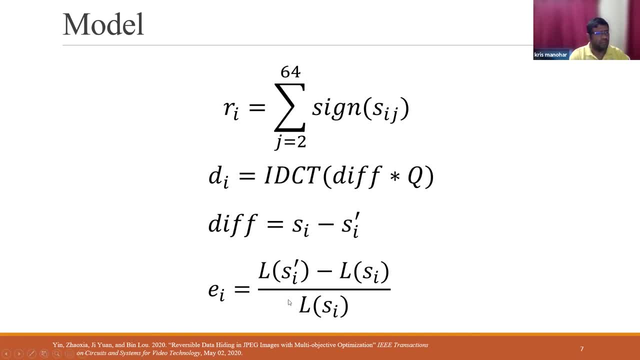 and get an idea of the length of that compression. So essentially it's just taking the difference and divide it by the original. So we sort of get an idea of the coefficient. So that's the percentage in terms of the file size expansion. 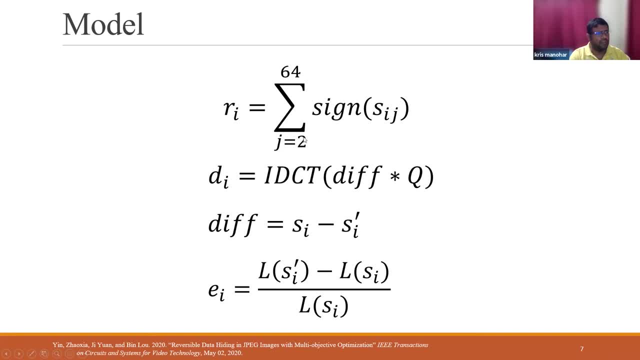 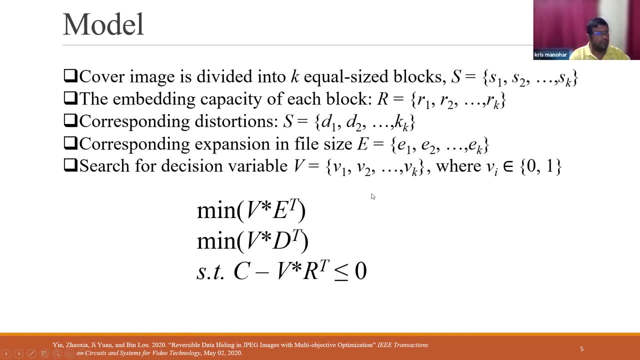 So they would do this for each block right, So for each component signal that side right. So they would do that for each one of those, And then that would generate the values for these vectors here, And then you just apply, I guess, any sort of optimization. 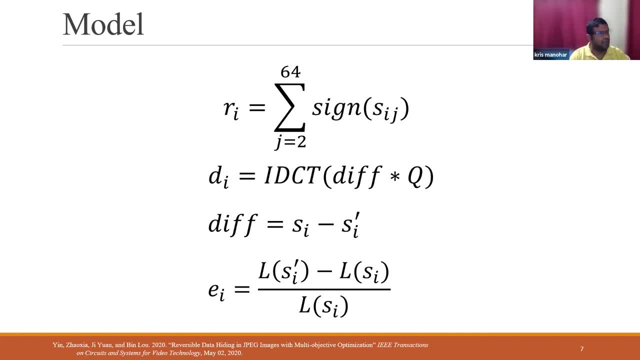 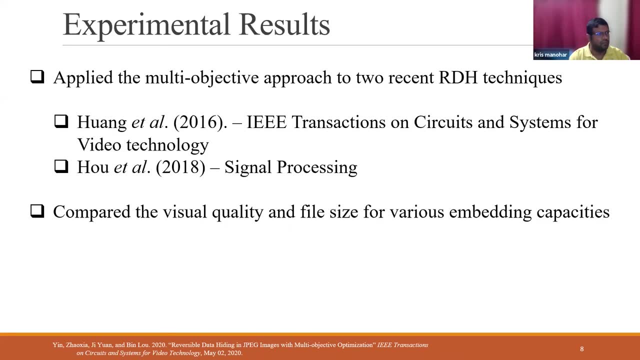 I think integer programming might work here, Because this is binary right: You just choose it or you don't choose it. So any sort of optimization solver could be the answer. OK, So that's the answer for that. So, in terms of the experimental results, what they did, 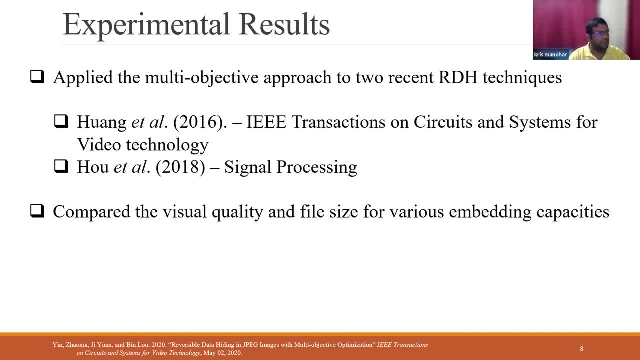 was. they looked at the two recent reversible data hiding techniques in the transform domain And they applied this methodology to it right. So again, the remedy methodology is given a particular embedding scheme. it would then be able to work out whether a pixel is embeddable. 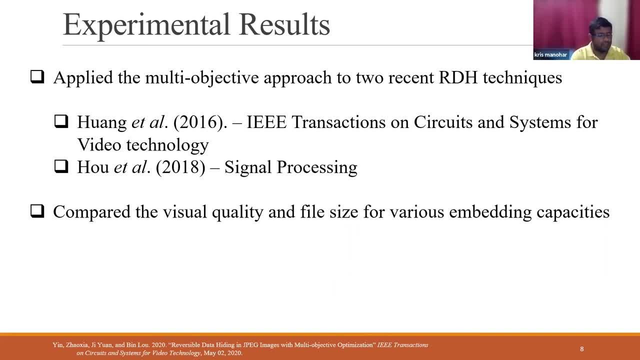 or not, by following that approach, And then they would fill that into the vectors And then they would try to solve for that decision, variable V, That is, the selected block right. So they would do that following these two embedding schemes by Huang et al and Hu et al right. 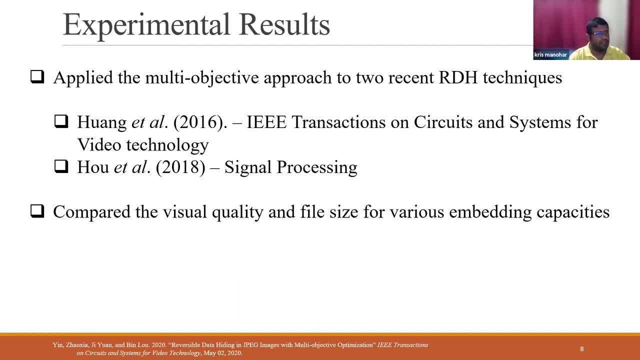 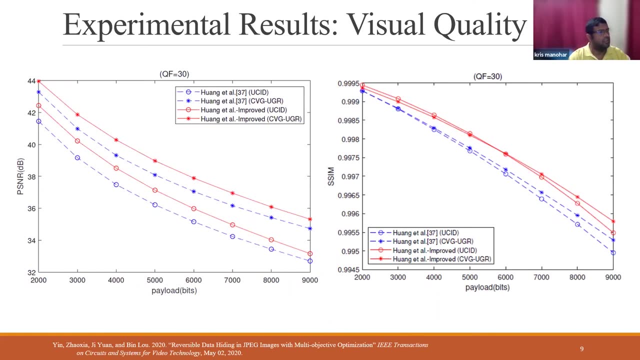 So after that now, they would then compare the visual quality and the file size of various embedding capacities where they followed their sort of selection procedure, and those by the original embedding technique, as proposed by the authors, right? So this is just some graphs from their paper. 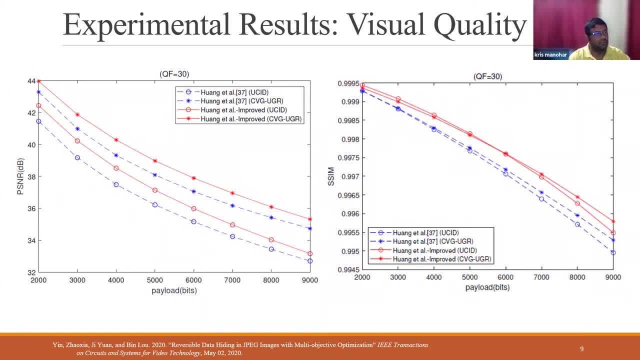 And that's a really, really Impressive result. So this is why this was sort of cool right, Because if you see, here in most cases they had like almost a 1.5 decibel increase, right, And so this quality factor here would be tied to a quantization. 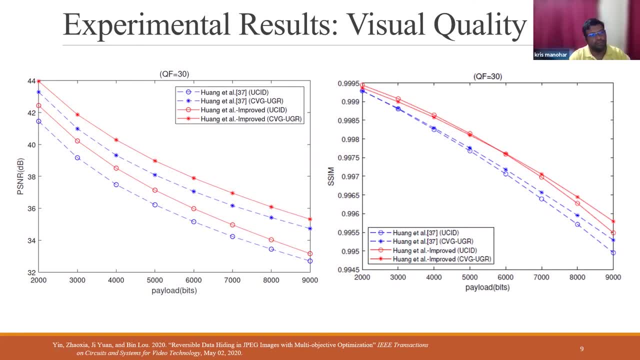 table, because the quality factor determines how much compression you want, right? So the higher the quality factor, the less compression. right, So the more original the image would look in terms of the raw picture, right? And if you have a A lower quality factor, then you're going to have plenty compression. 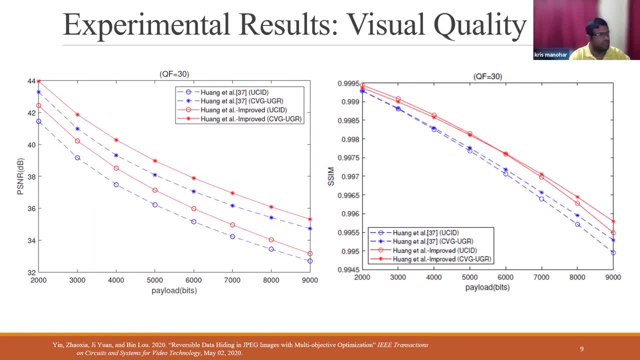 So you see more artifacts, but then you will have more redundancies, Right? so they compared it visually to the PSNR, right? So the distortion that they had computed was basically modeled after the PSNR. in terms of the PSNR is a logarithmic scale that measures the sum of the difference. 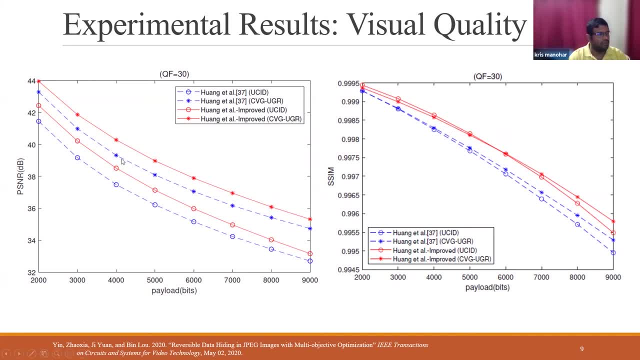 between the squares in the original signal and the stegosignal Right, Whereas the similarity index are the interesting, So the structural similarity measure here that they have. there's a formula that is used not to measure the visual quality in terms of how the two images look right. 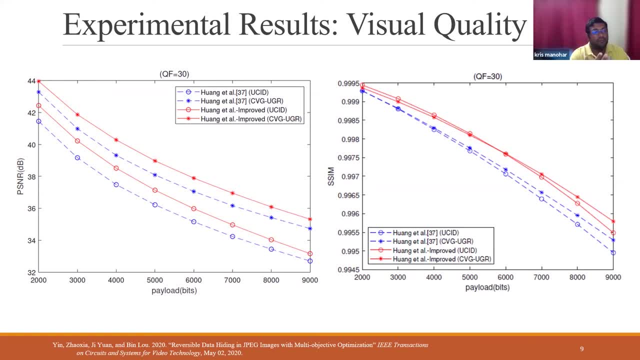 I mean, this is the ongoing year of research. How do you assess image quality is a big topic right now. right, So we have the original one, which is we just measure the distance in modified signal is away from the original, and then you have the distortion. 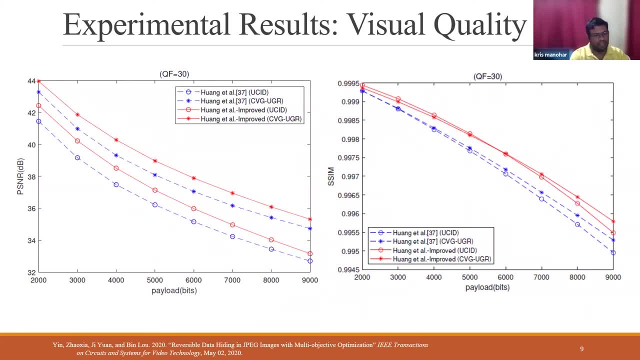 Right, structural similarity, where it sort of tries to give you an idea of if the information content is similar in terms of how we would perceive it. you know the lines where we expect to be lines, they are lines. they are no sort of blues. So if we have expected to, 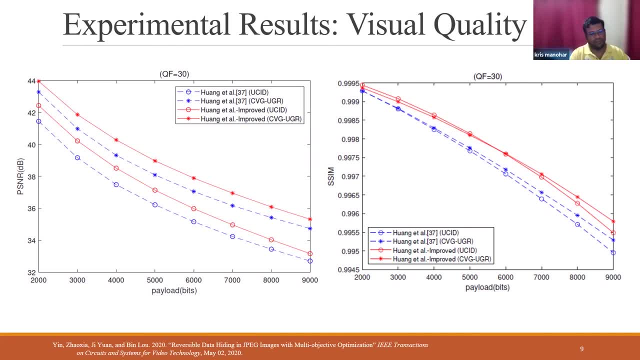 look like a road corner. we do expect it to see sort of jagged off the end. we expect to see nice straight lines. So the structure of the image is sort of consistent, right. So you see, for these smaller embedding capacities, right, it was more or less identical. But 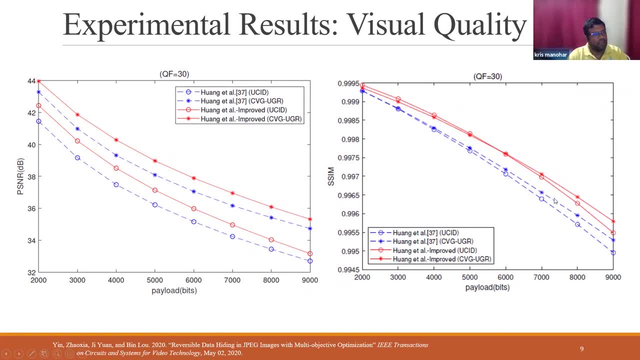 then as they come down here, you know we start to see a huge divergence in terms of the structural similarities. So the higher the value is closer to one is, the better the similarity right. And you can see here in the improved vision the proposed scheme was. 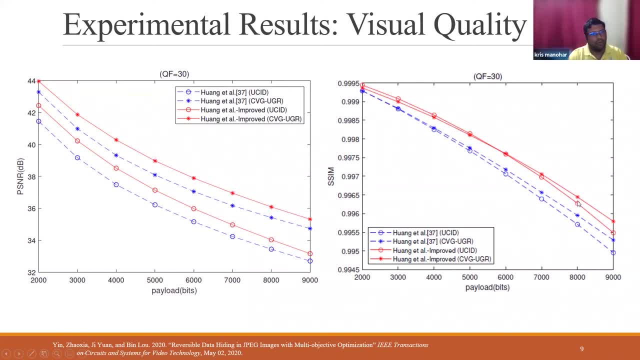 able to better select the blocks right that cause distortion. but it also- you know what was really interesting, was it? It choose the blocks that are more or less identical, right. So it was able to select more of the bought blocks that are more or less identical to what you need to buy, right? 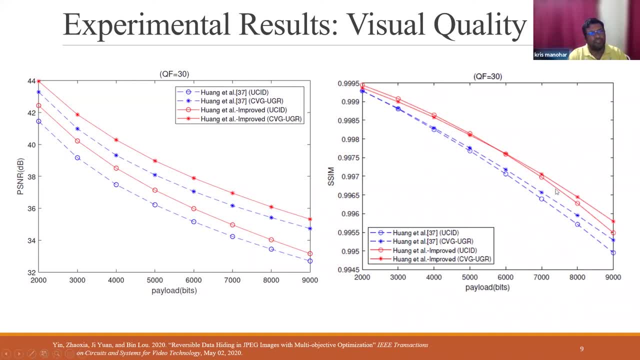 And it also it choose it based on this PSNR like thing, right, But it also preserves the structure of the image, And this was rather amazing to the others and to me as well, right, You know that it was smart enough to sort of pick the right blocks to modify so that 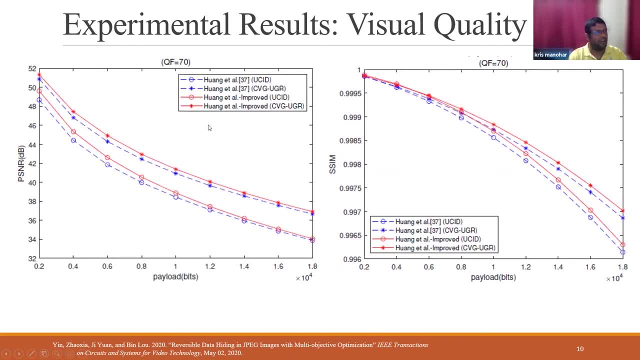 we wouldn't be able to tell right, And this sort of held across different quality factors. So again, as the information content increases, you know, there's less room for redundancy, right? all the pixels are sort of important, right. 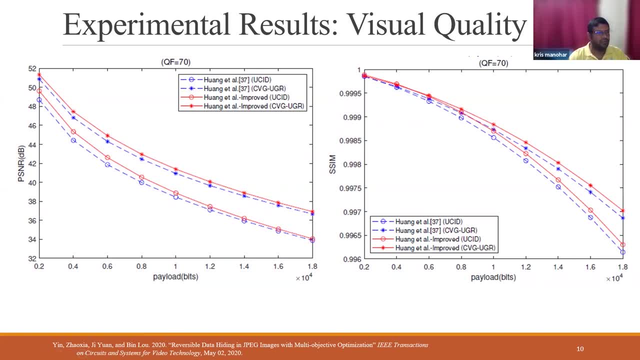 So as the quality factor decrease, you would have a lot more redundancy because you know compression right. But as you have less and less compression, the information becomes more and more relevant. So you would find here that the deviation between the improved and the original one 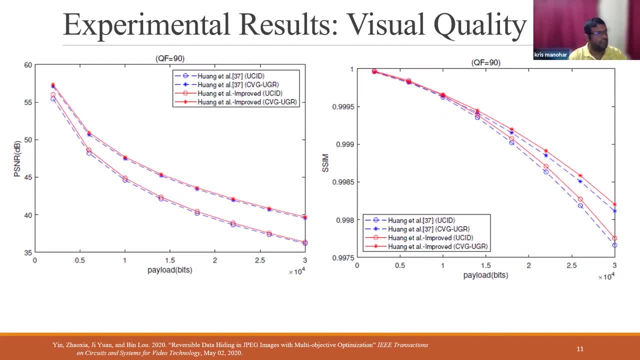 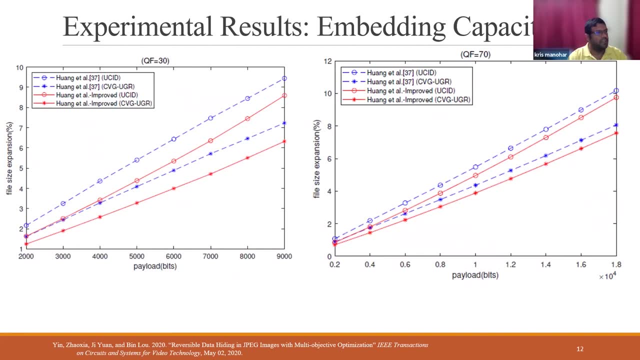 you know is sort of similar. you know, in that scenario, Right, And same thing as you were talking about In terms of the embedding capacity. what we found here was that this method was able to get a lower file size in terms of the different payloads, right. 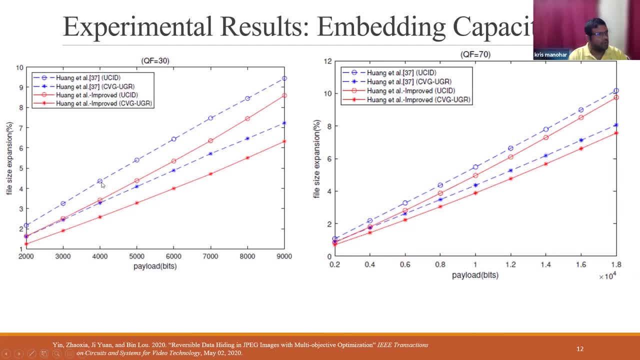 So if you look carefully here, we would see the improved one as the one with all the stuff Right. Yeah, that's the one with all the stuff Right. You would see the in terms of the file size expansions, it's really not that big right. 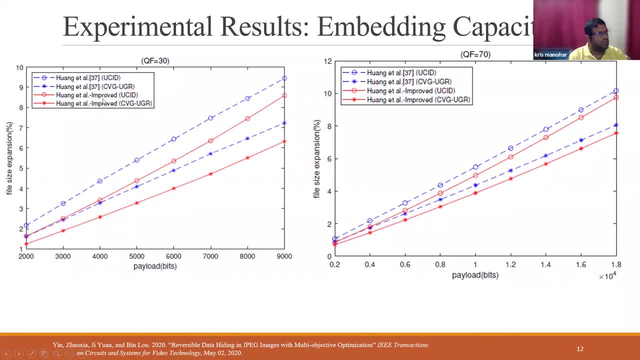 So the improved using the two different. oh, sorry, I forgot to mention they used two different data sets here: the UCI data set and the CVG data set. right? So when you look at it in terms of the file size expansions. 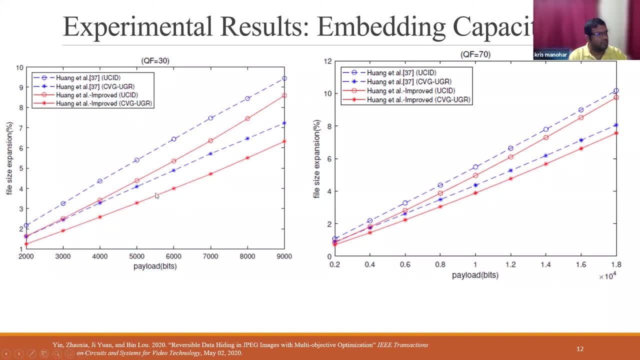 they really got some good results as well, right. So, as the payload increased, the percentage of the file size increase was decent, right, And this was a really really big contribution, right, And this was a really really big contribution right. 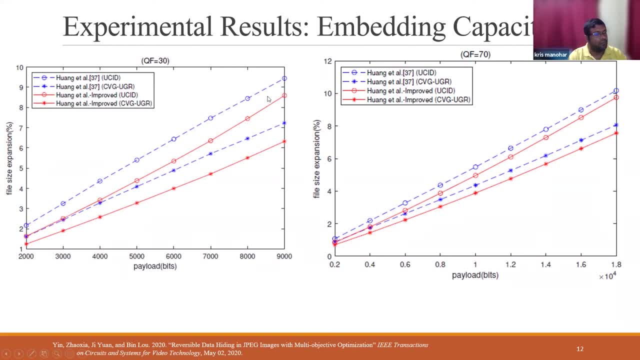 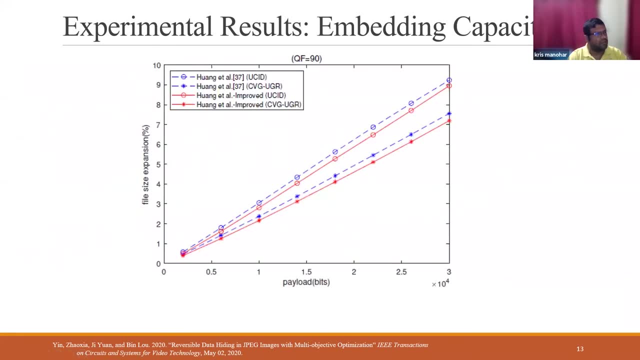 And this was a really, really big contribution to the field, because most reboots building techniques didn't consider this sort of approach right. So, and sort of similar results, as you would have moved ahead in terms of the quality part, right. 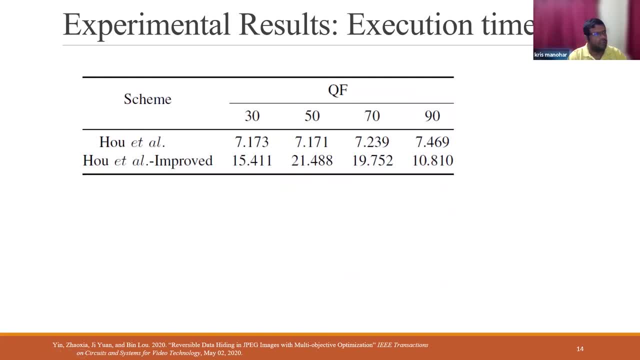 So, in terms of your runtime, what we found was that, if you would, this would obviously take significant longer, right? So sometimes you order like twice or three times as long, depending on certain factors, And this is because for each image, you would have to- well one- make the first pass. 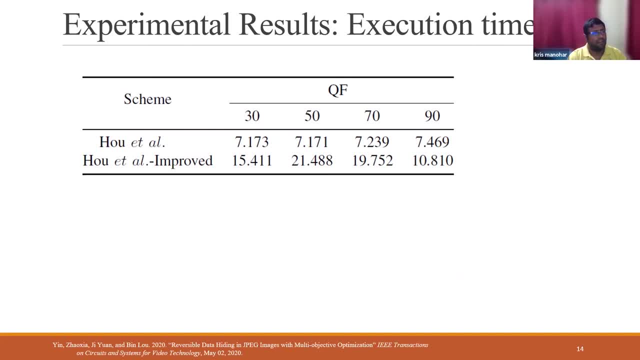 to figure out the values for those vectors And then after that, it would then have to apply the optimization technique to find the decision variable V that would minimize the different criteria right. So there's this trade off in terms of the runtime, which is expected because there's no free lunch. 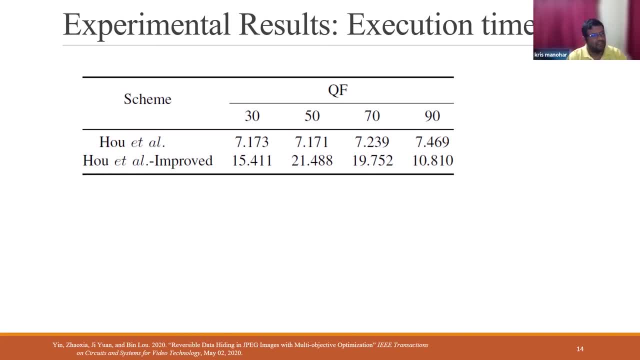 So, while the work is interesting, there needs to be some more, more improvements in terms of how fast this competition could take space, because I mean these in terms of the order of seconds, right, So you know if you're looking at us. 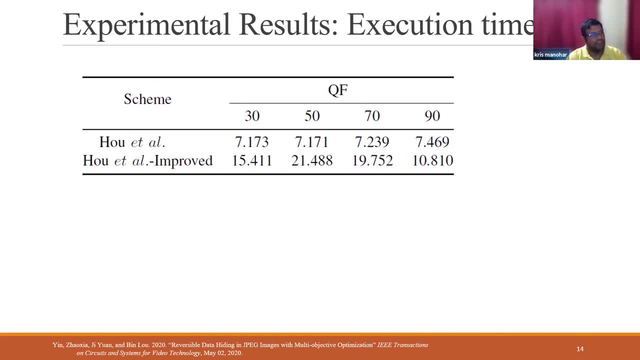 like a real-time system. so so, moving on from here, this sort of just optimized this on one front, right. So like, how can we improve? Well, you can think about trying to find the curve and the sort of optimization for the periphery of the. 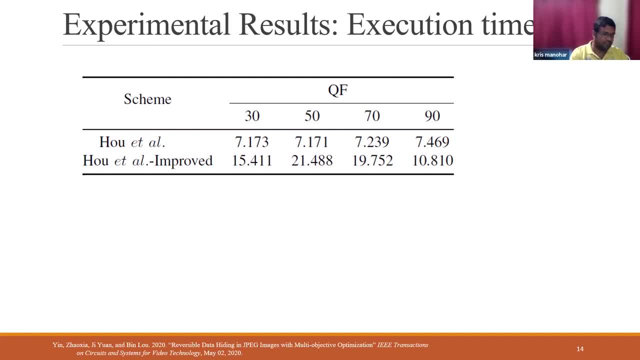 the the different objectives. So then we could actually quantify the actual trade-off between the visual quality, the embedding capacity and the file size. So you could think of all the application as someone coming in and saying, okay, I want to have a maximum, this visual quality. 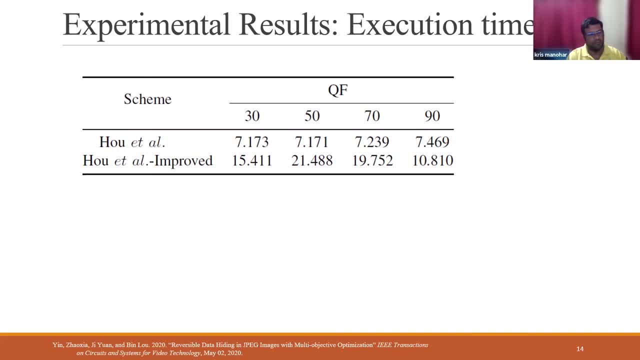 I don't want the file size to increase by this much, but I want to be able to embed 50,000 bits And then, once you have that curve, that outside of the curve, then we could actually scan it and see if that is a possible point. 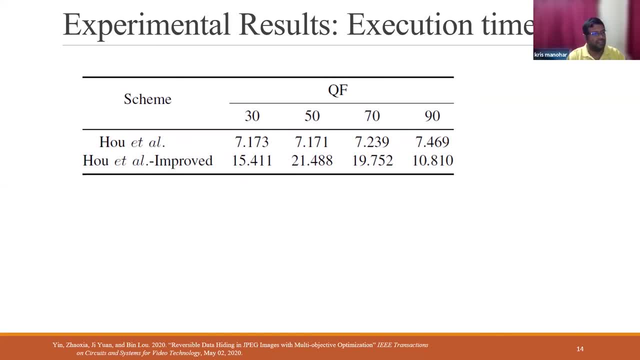 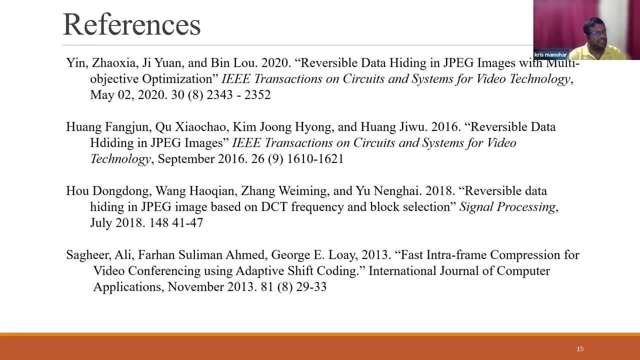 that could be facilitated by a particular image, right? So that's the next steps in terms of how we plan to sort of improve on this. So that's it there. Dizzy, These are references. yeah, some really, really good work.